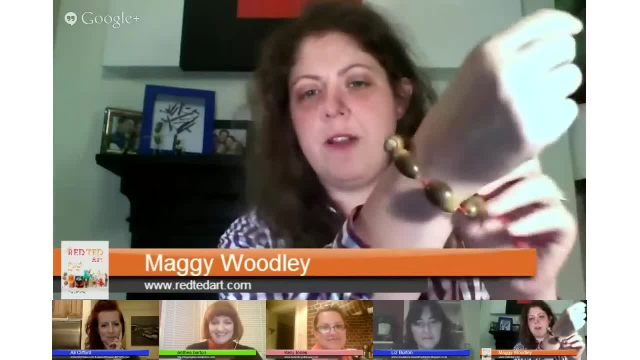 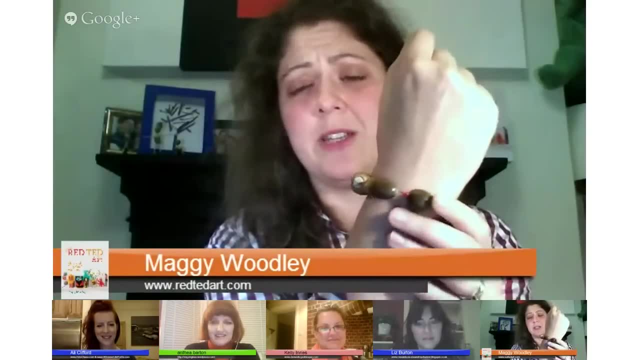 So my focus this week was actually acorns, So my very first one is this little, super simple acorn bracelet, Really really easy to do. Obviously you have to do it with the kids, but like a lot of these crafts, I think it's fine to do it with them. They enjoy the process of just 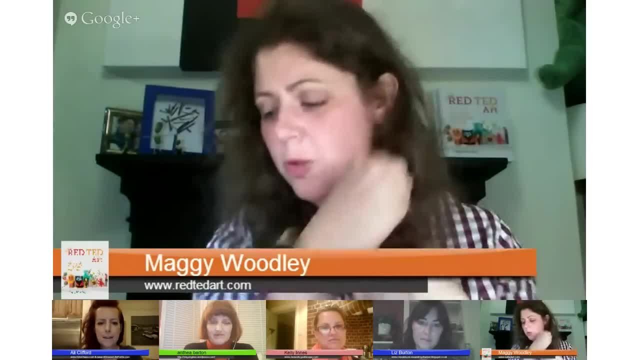 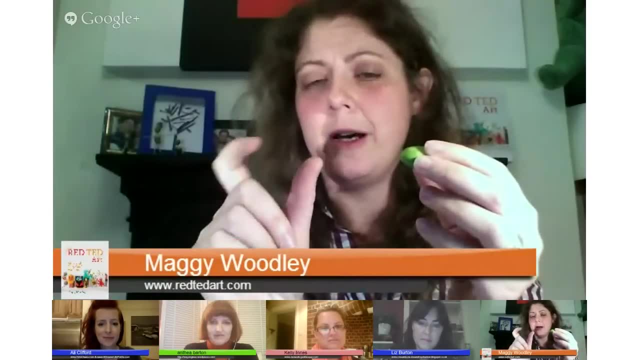 sitting down, sort of selecting, sorting and seeing what they can do. So all you have to do is you take your acorn- We call these little hats- You take the hats off and then you have to get a really big needle with a big eye, So one that a thin ribbon will fit through, And then you push it through. I found it. 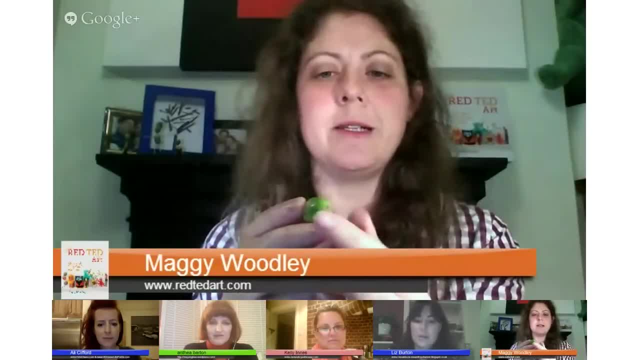 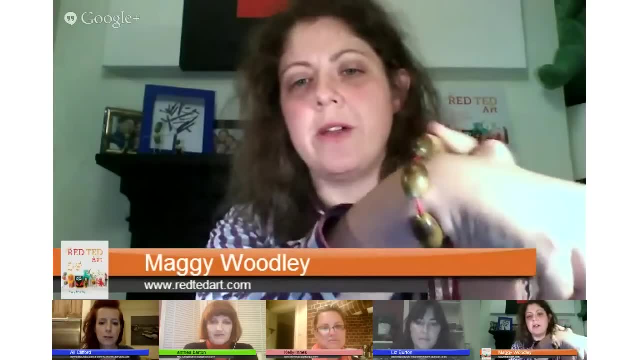 easier to start at this end and then poke out the other end. And if you start with the green acorn, they're a bit softer and easier to handle And then over time they'll go brown, which is quite fun in a way, because you start off with a green bracelet and about a week later, or two weeks later, 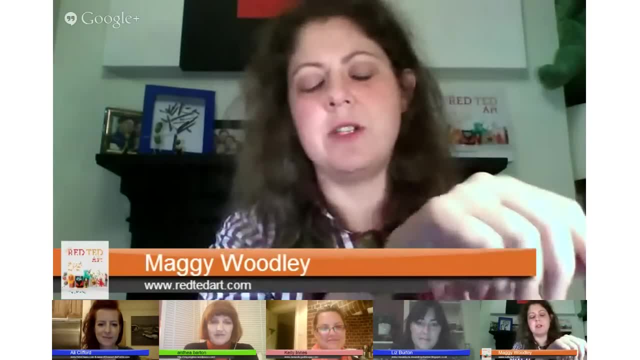 it'll be brown And I think that's quite sweet And you can do necklaces or whatever. So I thought they were quite fun, Really really simple to do. So that was my first acorn. So, seeing as we took, 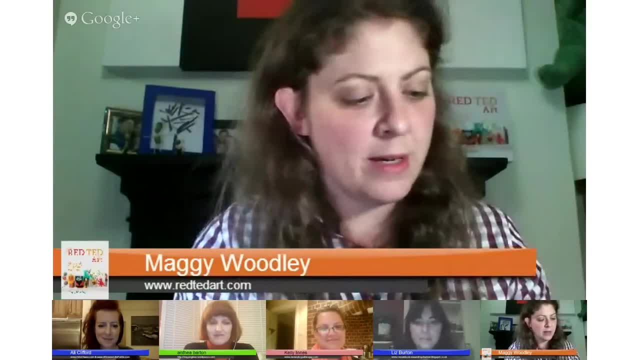 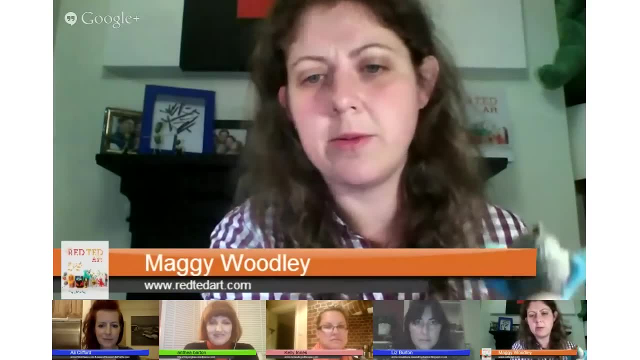 the little hats off. what do you make with the little leftover bits? This is a classic craft that you've probably seen already, But obviously we had to do it because Pippa loves all things tiny. So here we go. What is it? Let's see A little teapot. So we've got a little acorn teapot. 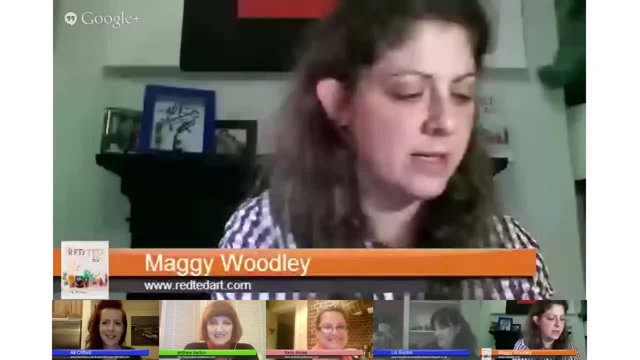 that you can open and then you can fill it with something, And here's a little teacup to go with it. So I made a little, a whole little set. I think people have made them a little bit different. I've got a little teacup that you can open and then you can fill it with something, And here's a little. 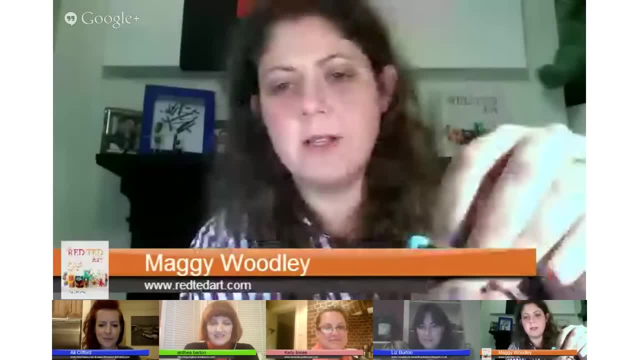 teacup to go with it. So I made a little, a whole little set. I think people have made them a little teacup to go with it. So I made a little, a whole little set. I think people have made them. 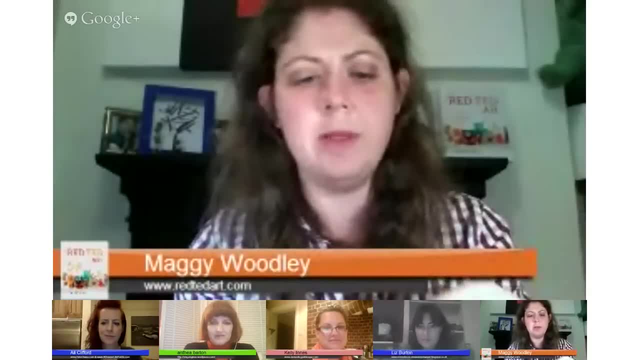 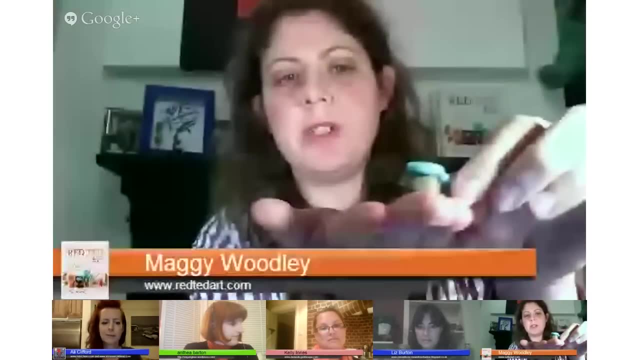 in different ways. We chose to use Fimo, the polymer clay, And basically I did the little shapes. I dried it in the oven upside down like that, And then afterwards you can see I use a hot glue gun just to secure it. I was going to use super glue but I couldn't find it So hot glue. 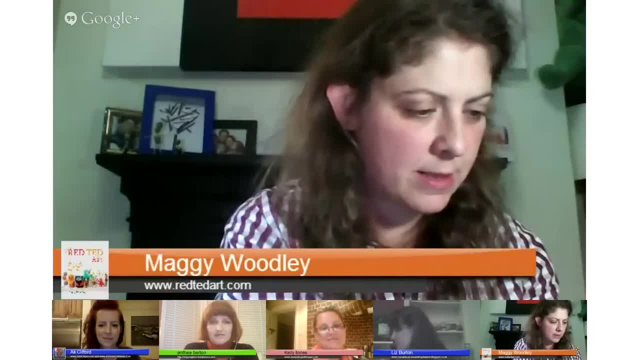 gun it was, And we did a little, so we've got some teacups. There's a little. where's the milk jug? Oh, there was a milk jug, But I think my favorite really is the teapot. I just think it's so cute. 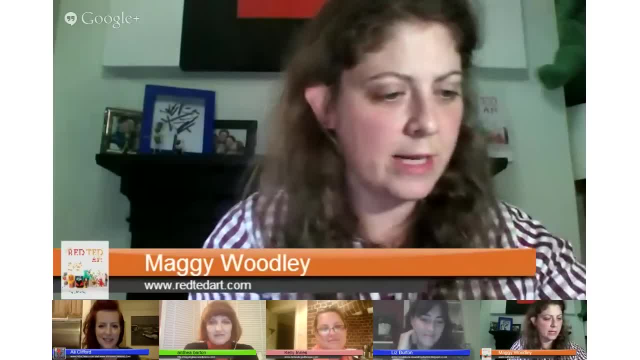 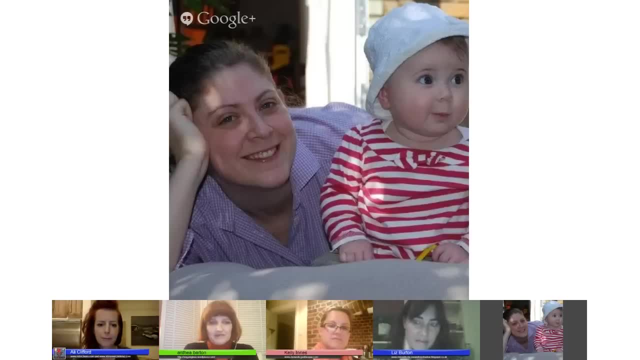 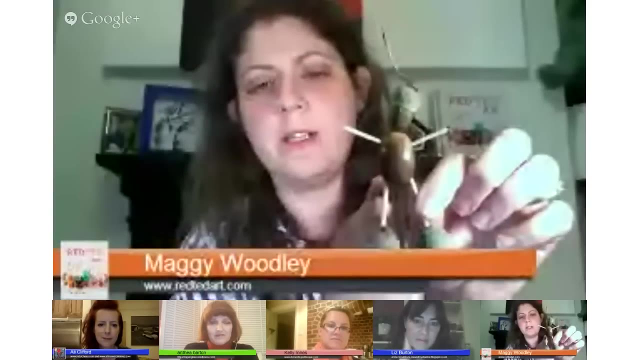 So we've got that. So that's acorns, And then, oh yeah, the really obvious acorn one. It's a classic from my childhood. Here there are these And two pigs. Two pigs. We've made them with twigs before, which I think looks really nice. 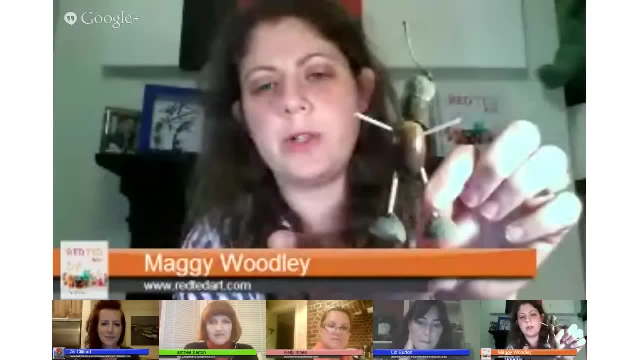 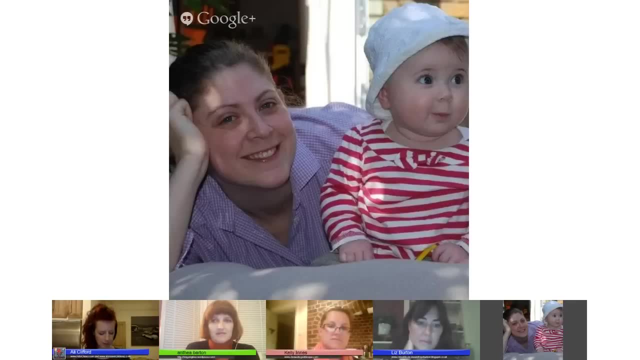 And this time we put on some little cat balls. I just love doing these, or doing these little animals. So here's one, Here's a little horse, And this, to me, is classic autumn crafts. I mean, this is what I remember about my childhood and I absolutely adore it. 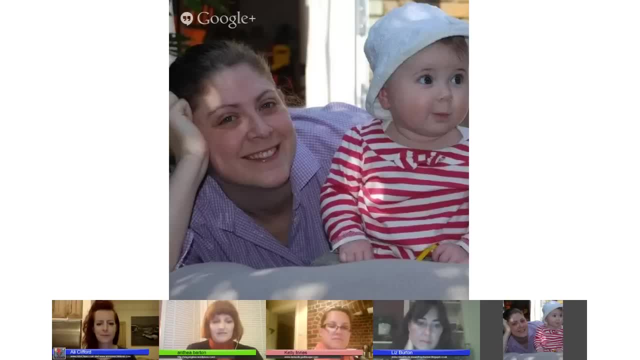 And as we're expanding on that a little bit, whilst the kids were fiddling with theirs and trying to choose what they wanted to make, I suddenly realized that I had this little poppy seed husk. Here we go, She's coming. Oh, here's a poppy seed. And she was a perfect head. 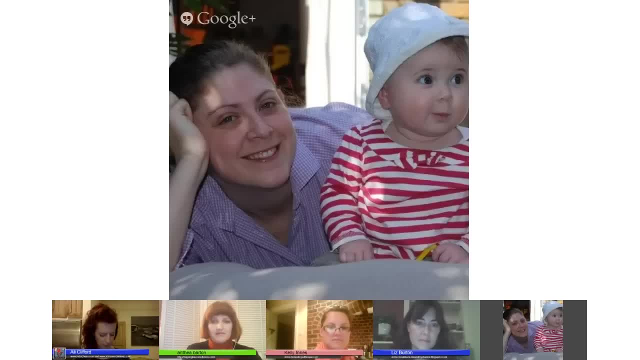 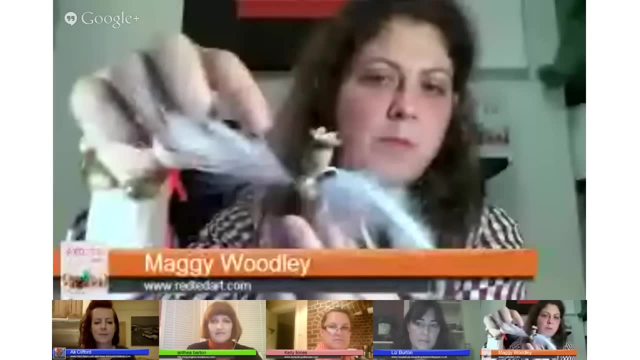 And we picked up some feathers and an acorn And basically I made a little hole at the top and then shoved the poppy seed husk in. with a little bit of glue I did a tiny bit of glitter, some sparkle glued on the feathers and we have a little angel. So those are mine to begin with. 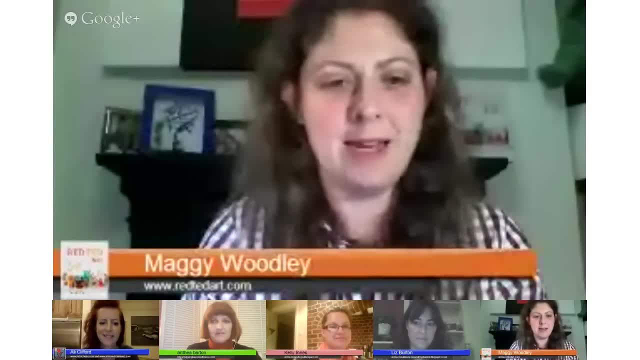 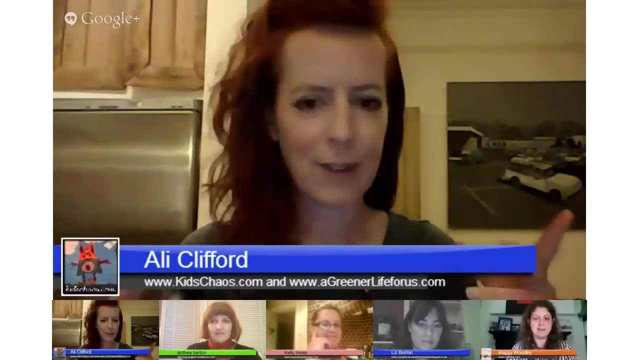 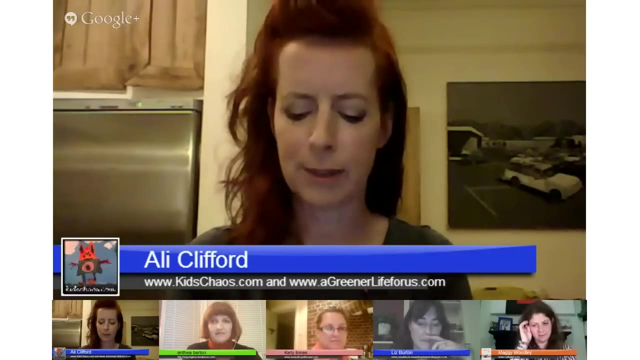 I'll bore you with more later. I'm going to pass over to Ali now. Evening everybody. Hi hi, hi, hi hi. So mine's fairly simple and quite quick. It's printing with leaves and with their own natural pigments. So we picked some leaves up just from the back garden. 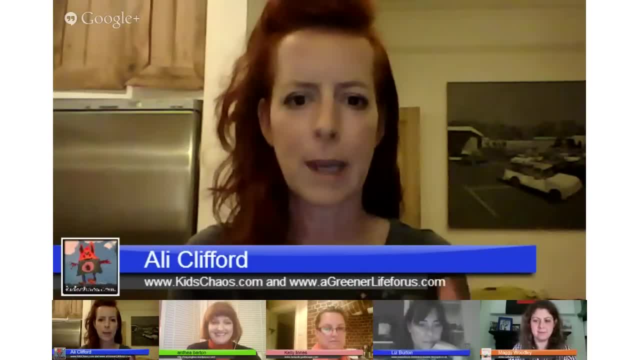 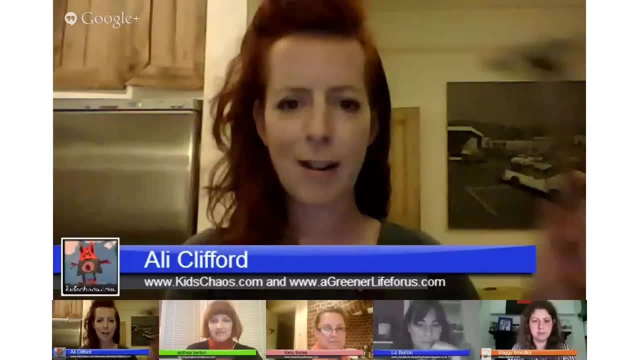 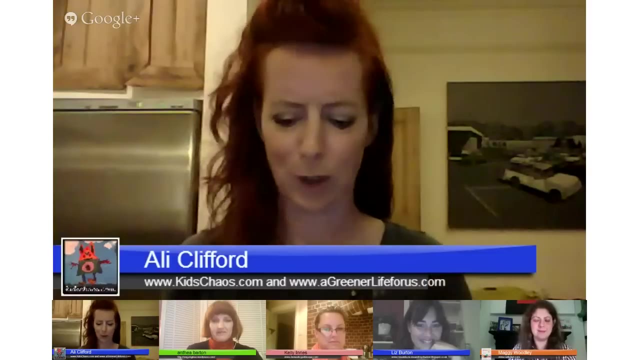 and you need some good paper, like a really nice watercolor paper, a couple of sheets of kitchen towel or kitchen roll, a hammer and something like a chopping board, so that you're not hammering straight onto the dining room table, which is what people want to do. And it's amazing You've had a couple of sheets of. 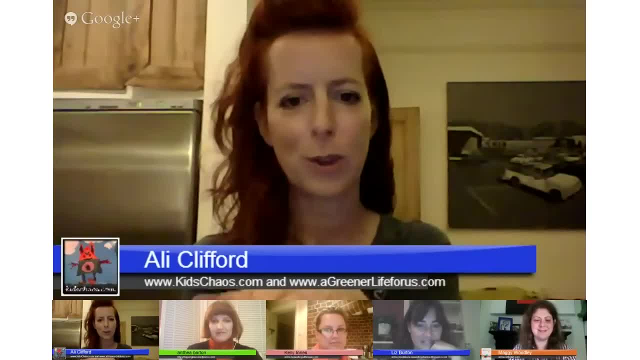 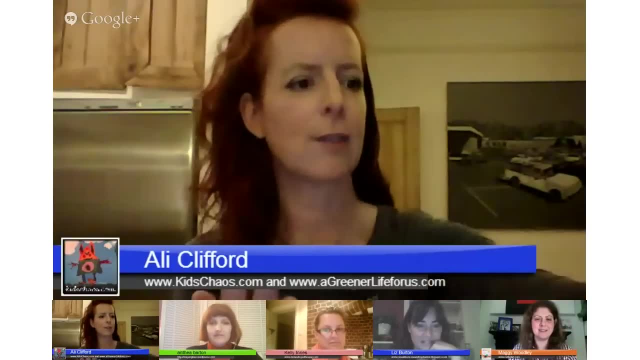 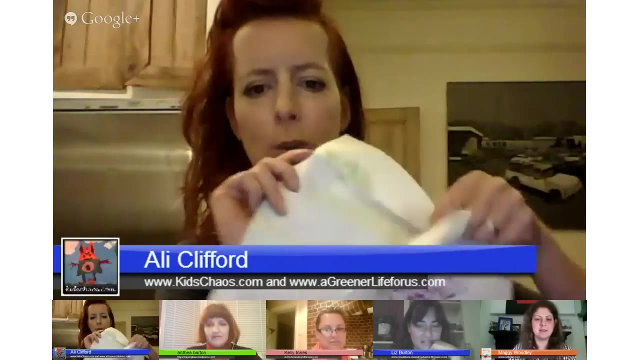 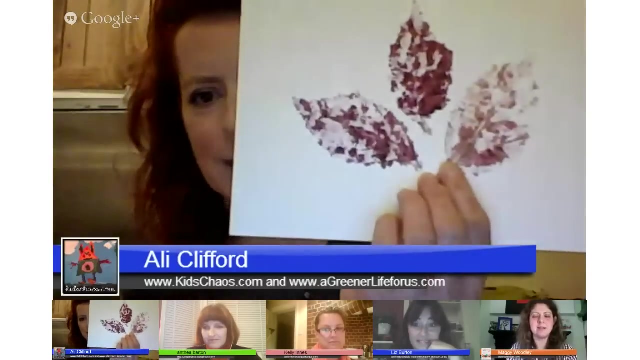 paper, the kitchen paper- onto the leaf and just hammer onto the area of the leaf And it's amazing. You can see the pigment start to come through on the kitchen roll, and that's when you know when it's working. And then look at these Amazing, Beautiful prints. This is my favorite one, which is: 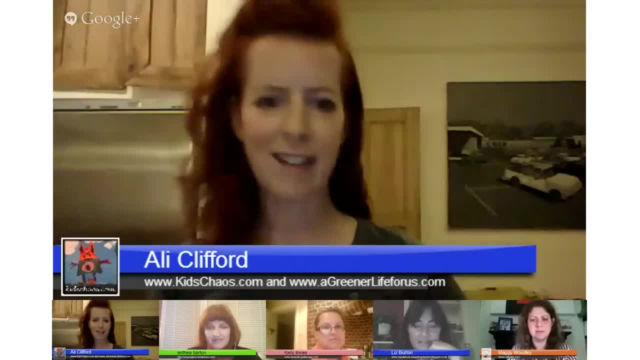 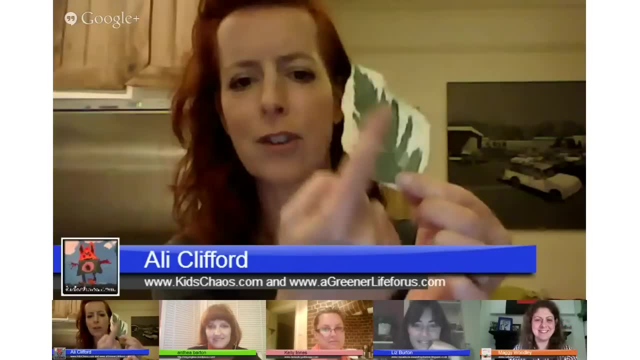 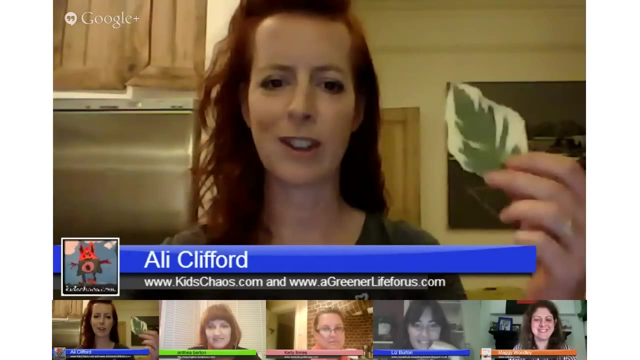 see the green, this one here, which was the variegated leaf. and what was really fascinating about that- well, for me and for him, was that it only really took the dark area of the variegated leaf and not the variegated leaf, And we've now got the one. that's even more beautiful now. 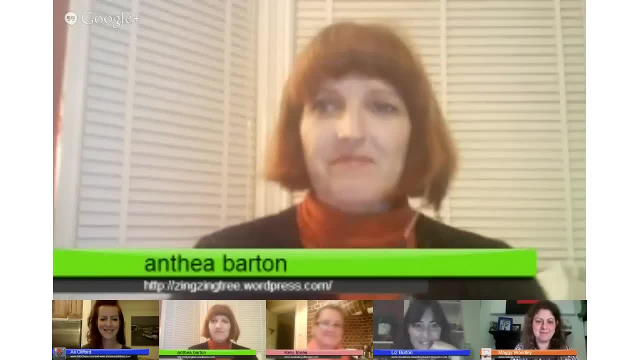 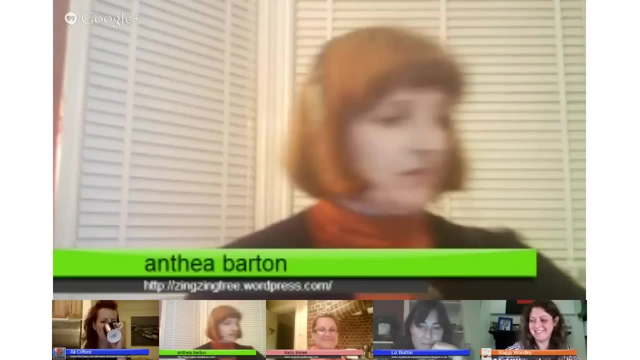 and it's a very unique, beautiful piece. I've never seen anything like that before. So all these are my avocados and this is my first apricot and I've always loved to and was really excited to see how they look after the shoot, So we've done a few of those. 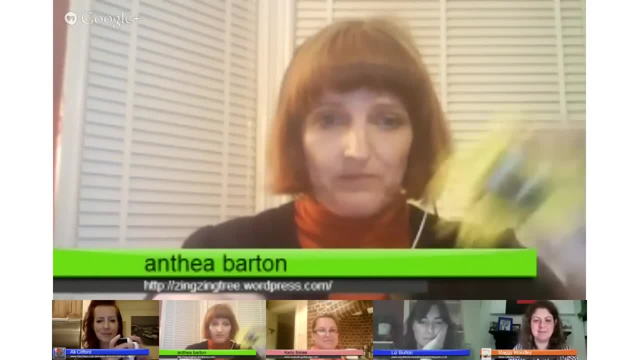 We've done a couple of very nice activity pictures and we've got a little bit of an upholstery here. we've got some wildflowers, some wildflowers, and we've brought some hollywood, some wildflowers And the dry leaves, lots of beautiful little green樹 leaves. 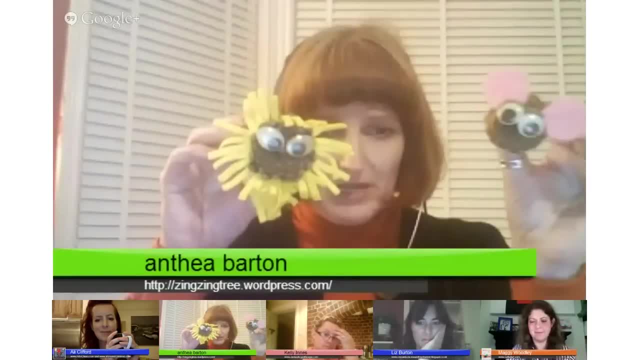 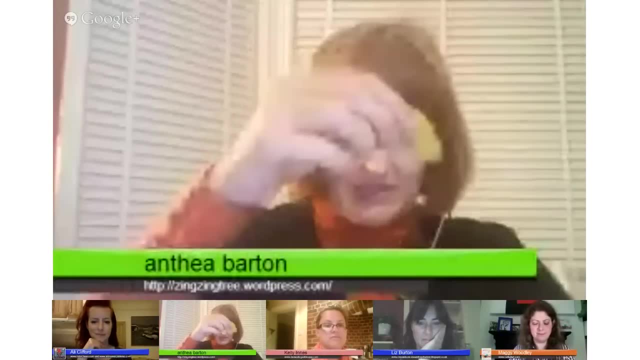 and the other stuff we've got is this little tree fabric really, or you could use paper and you create little beasties, so we've got you just kind of. you know it's nothing, nothing fancy, so we've just got this. you know, cut whatever shape. 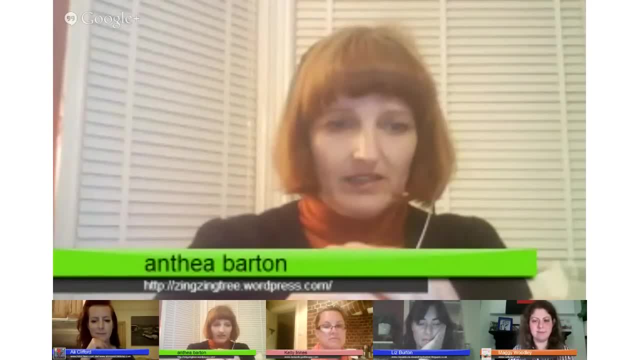 you are and the kids can just slot them in and they're quite good actually, because you can take them out and about. so if you've got a handful, if you're going to a wood or something, you can take a bundle of felt offcuts and the kids can kind of play around and make their own. 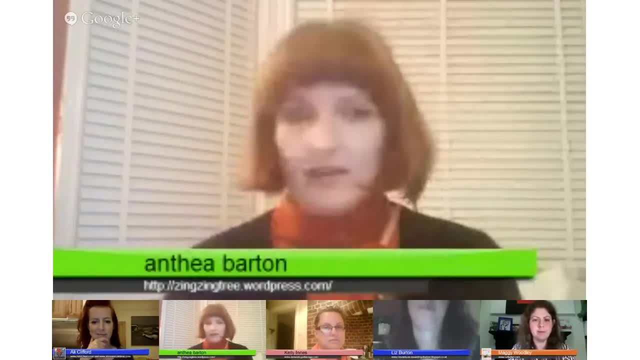 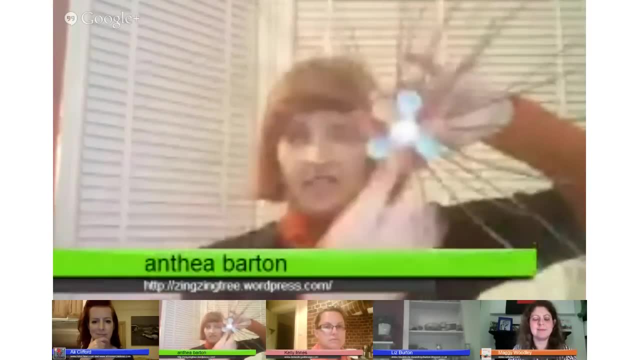 little beasties, and the new thing I've been playing with is twigs. well, actually it's not a question. I'll show this as well, because this is this is one I did earlier in the year and this is just taking a little bit of modeling material. so this is some model air, but you could use. 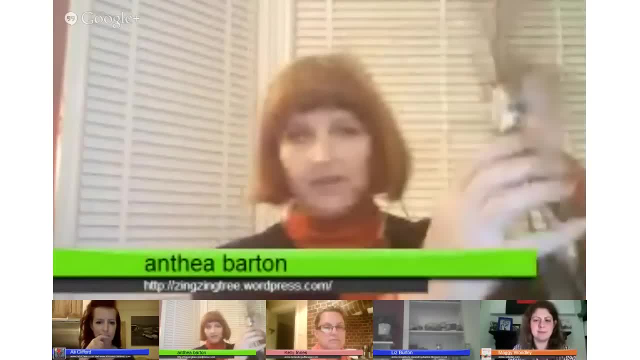 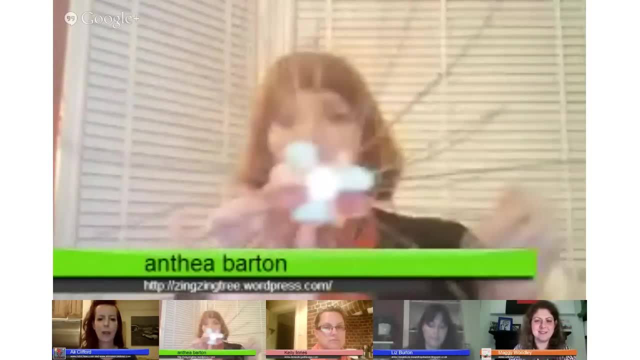 plasticine, you could use salt dough and then you just whack a load of twigs in that have fallen off the tree. so we've had lots of winds, so put those all in around the back and I've made some very simple felt flowers. you stuck those in just where it joins because it neatened it up. but you can kind of take this: 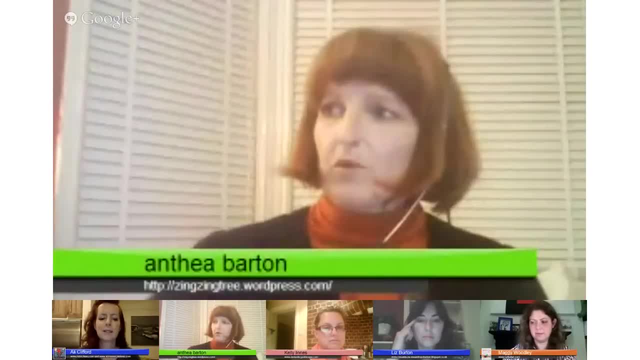 concept and you can kind of I mean I hang this on my wall but you could make all kinds of the kids can do it. they can kind of stick and create bugs and beasties and you can put googly eyes in again and you get a little bit more fun. and today I've just been doing something really simple actually. 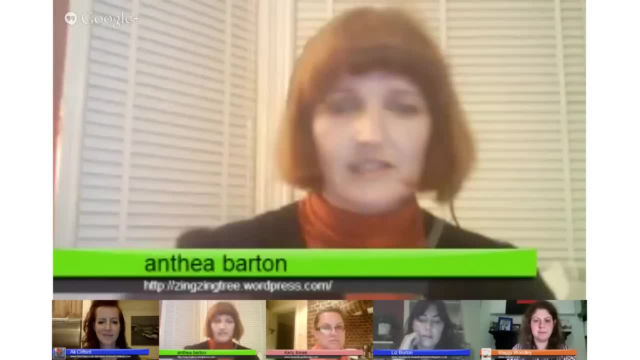 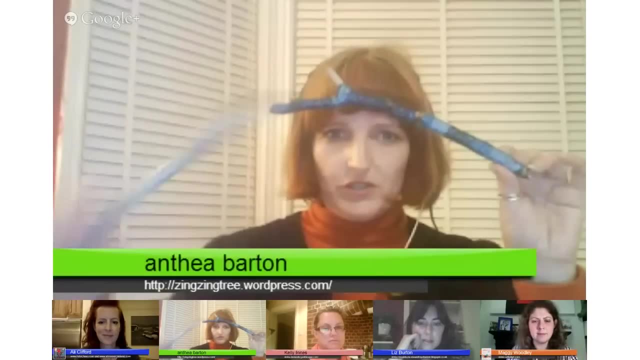 which I quite like. I've been wrapping or I might show. let's see if you can see. I've been wrapping twigs in wool but kind of I've got this new shiny wool that's kind of like a mesh and I really like here and I've just been just at 2 and I've actually got them bid as a center. 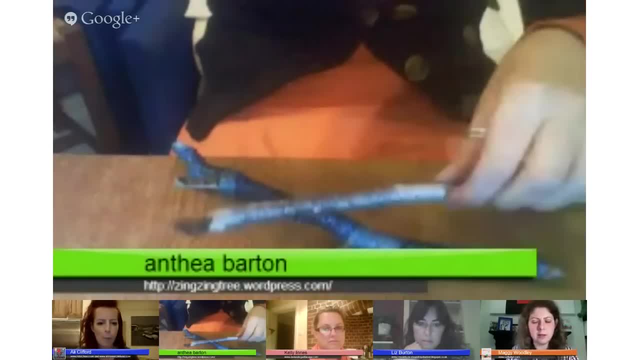 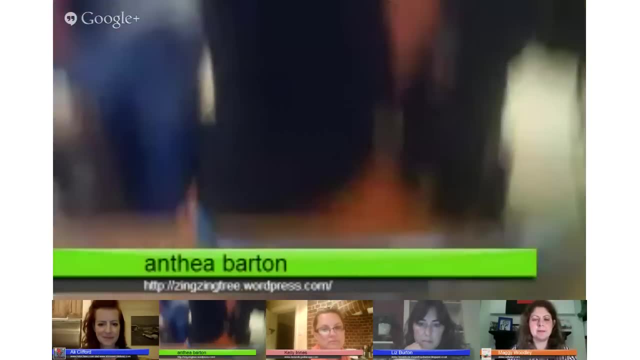 if you lay them on the table, it kind of quite good as just all the mental bits. we can leave them. not that you can add a a natural to begin, just a little bit of variation. stick them on the ball with my will. this is a little I've. 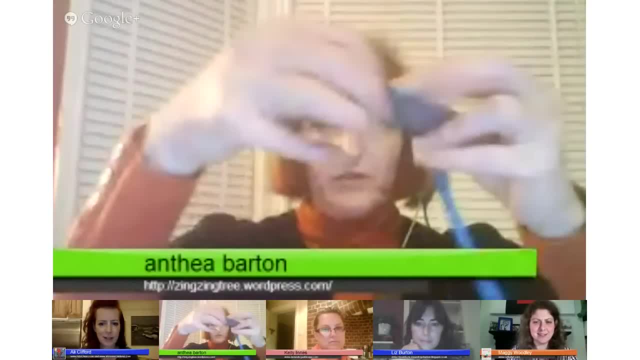 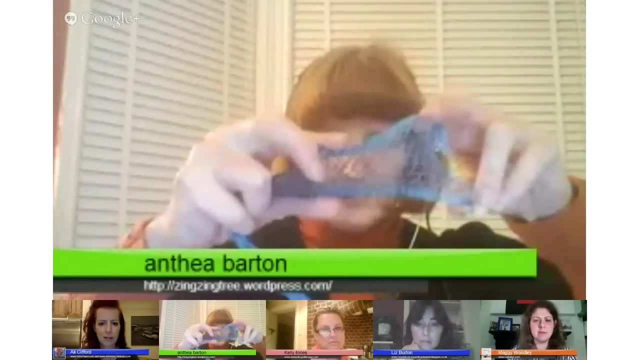 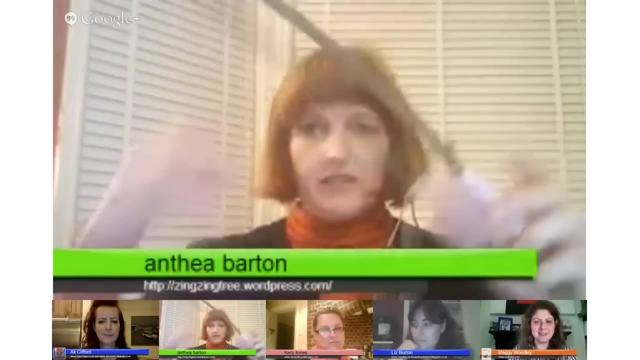 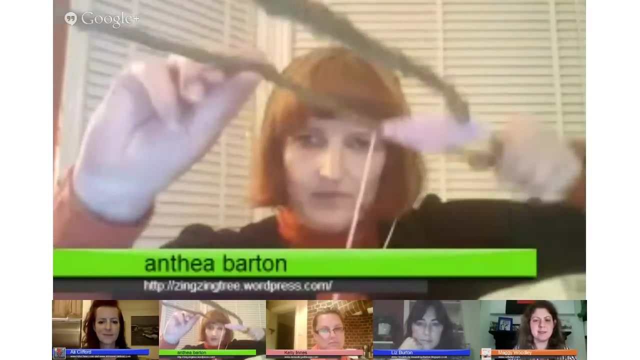 been using is this: it's kind of like exposure cable, so it comes. I brought it to some crafting with cuz. I like this to collage, but it's quite speak. you can make scarves and things with it. but it opens up. And then the other thing I've been playing with, but it's a bit time consuming, but I just thought I'd show you. the concept is when you get a twig or you could even get a branch that had three or four and you wrap the wool around it, so you get kind of like a ooh. can you see that? 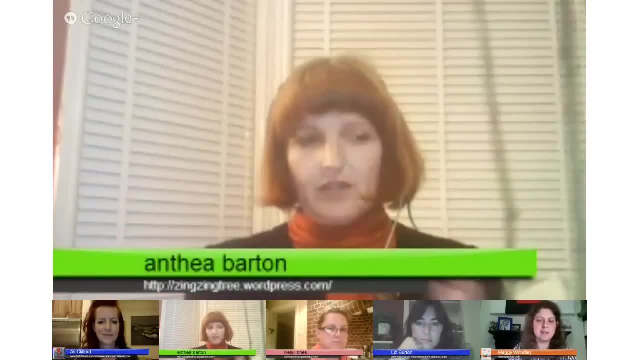 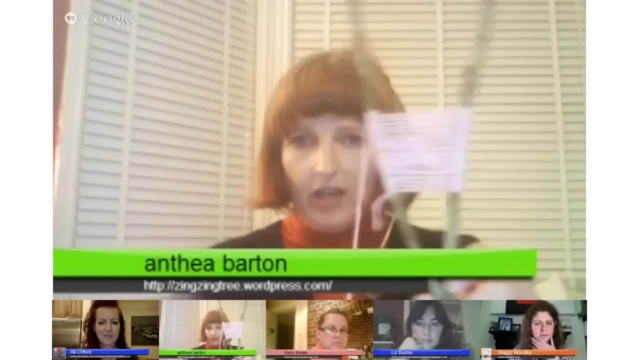 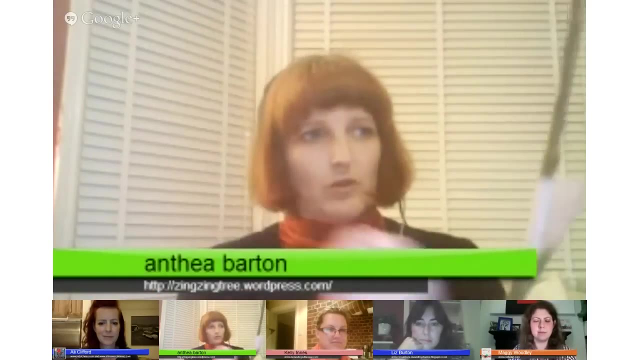 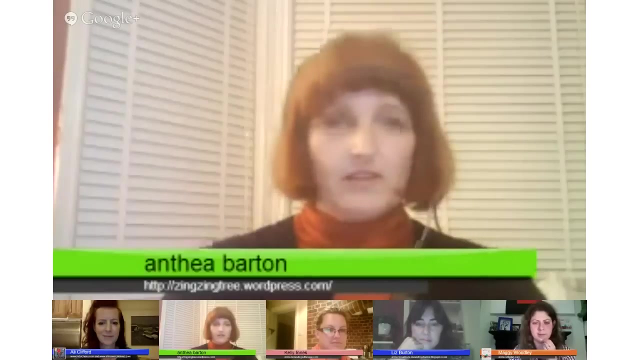 You get a kind of 3D structure. so you could actually have some fun. if I had some other twigs, I could wrap different colours and create almost kind of like a bit of an installation, because it gives quite a nice effect. so I've used quite a natural colour, kind of a pastel pink here, just to kind of keep with the wool. so I'm going to have a play with this and hopefully hunt in the garden and find a better twig and come up with something a little bit more structural that I can show you on the blog. 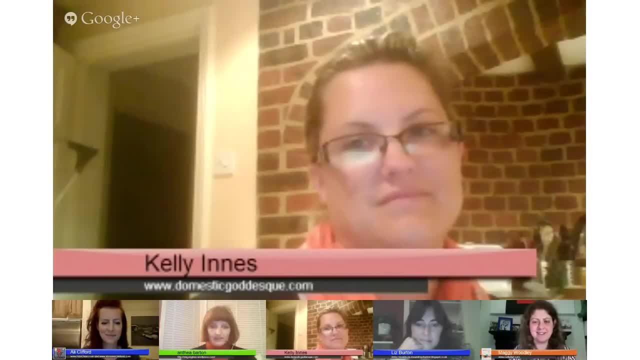 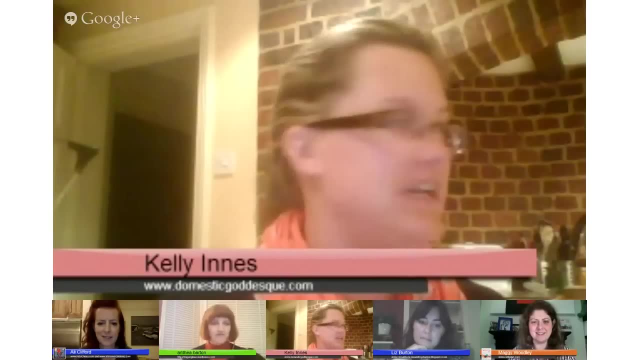 Now I'm going to pass it over to Kelly. Thanks, Anthea, Our craft. well, there are several. hilariously, I have very few of them with me. The first one that Maggie has. you're going to hold up the picture, Maggie. 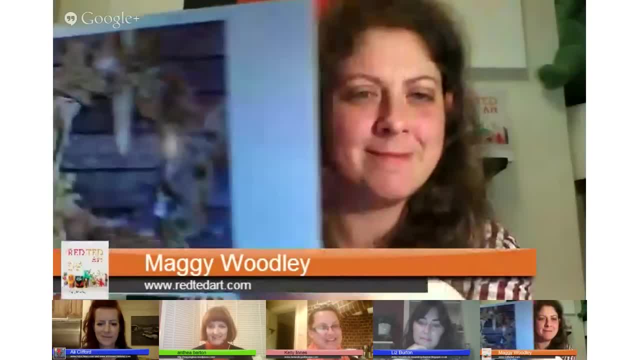 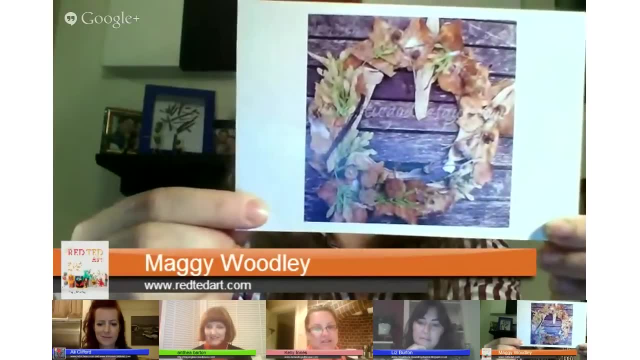 There we go. see It's on the blog, so don't worry. but round about this time last year, Dimples, who was then two, and I went out into our garden and obviously all the leaves and the bits and pieces were falling off the trees, so we did a whole kind of nature collection. 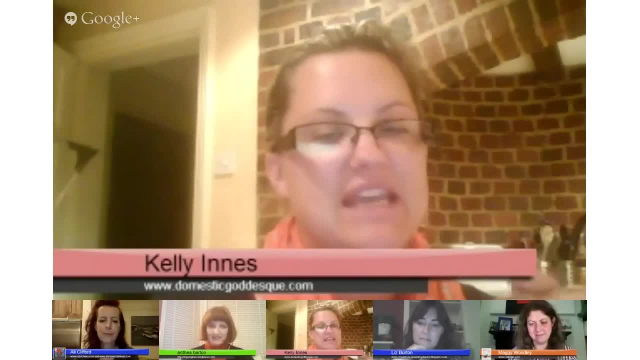 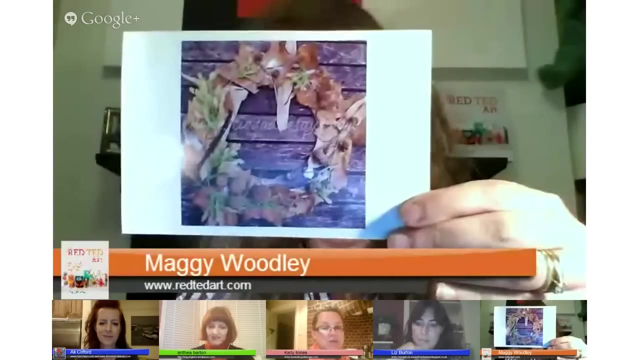 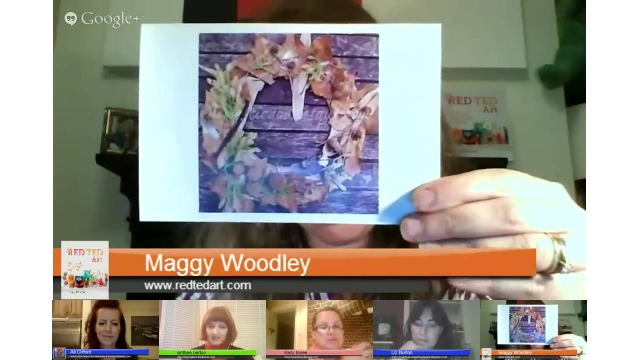 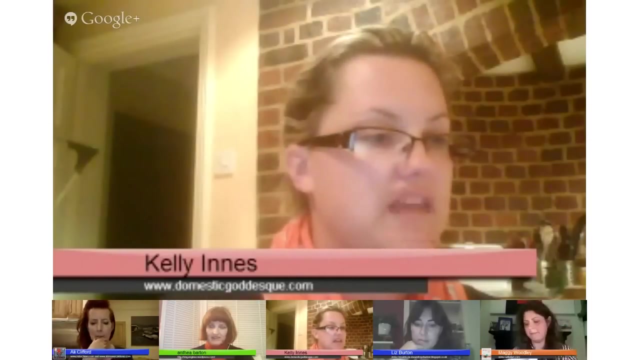 and we brought it back into the house And We made a nature wreath from it. I actually used an old cork placemat and I cut it out with a kind of craft knife to create this sort of wreath shape and then I just left her to it and she did all the sticking and all the gluing and what have you, and it was a really great thing to do. it was a great way to occupy her time, obviously, but also I think she really enjoyed sort of sitting down and working out what she could wear and stuff like that. so very simple craft to do for any age. 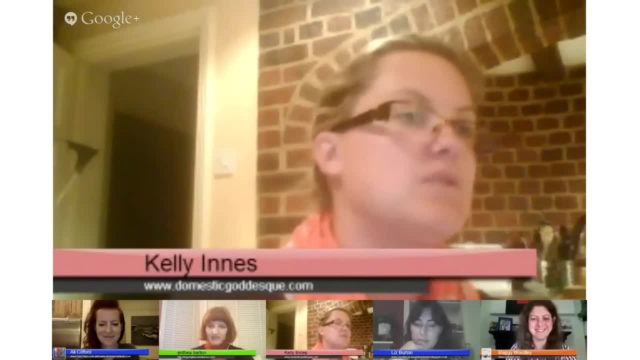 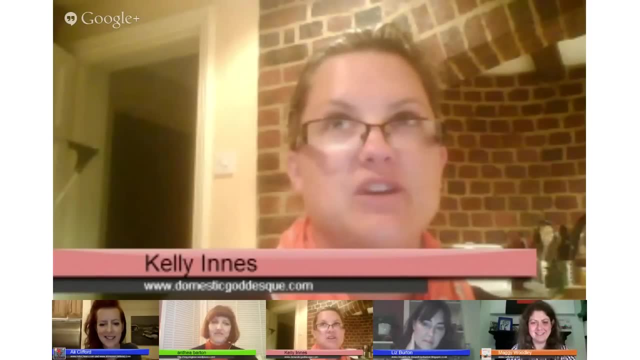 And second thing I have, which again can't show you, is: we just moved house. We've kind of acquired a bit of woodland And so we have lots of sticks and leaves and that kind of thing. The other day my husband very helpfully, when we first moved in, told the children about moles and badgers, and subsequently my five year old refuses to go anywhere near trees for fear that a mole or a badger is going to get hurt. 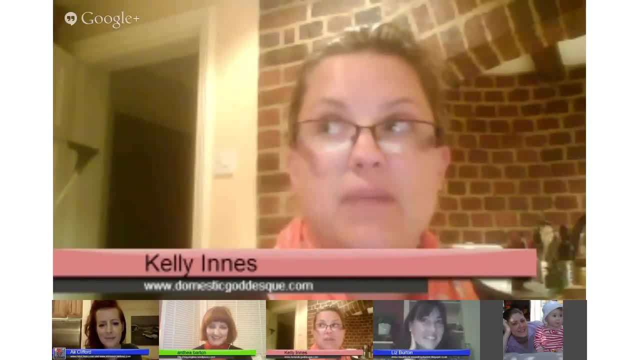 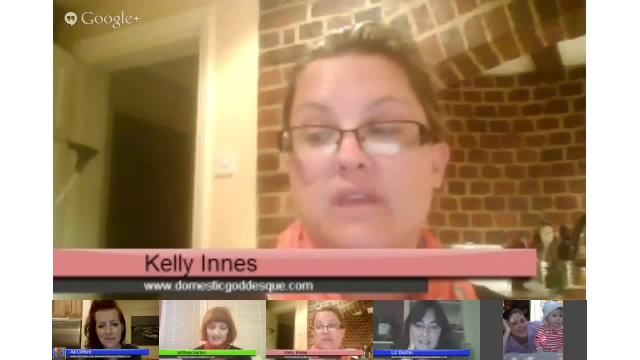 just so that they could put a face on it. And then, with double sided sticky tape, we stuck leaves on the back to create wings, and we are working on using those to ward off the evil badger and the woodland spirits that she seems to believe are out there. 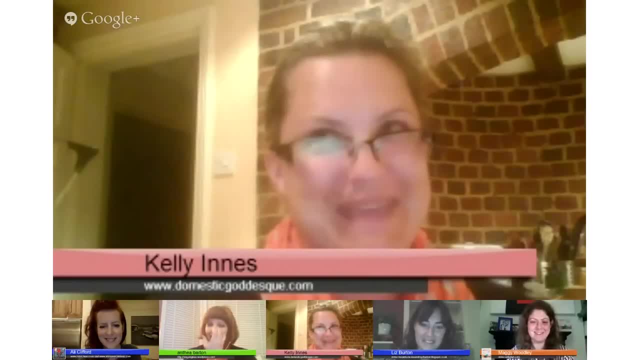 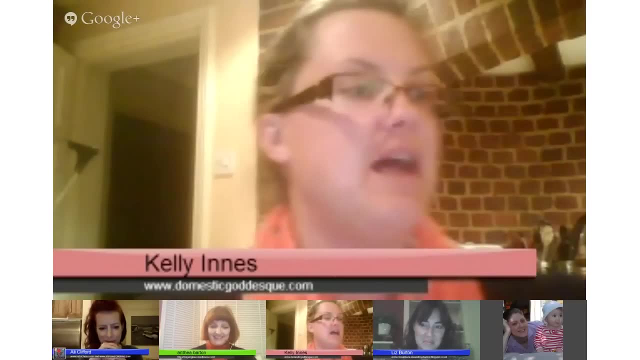 The reason you can't see it tonight is because she's actually taken it to bed with her under pain of death. Am I allowed to remove it? So that's that. But the third thing which I will show you- and it's very, very hard to see it- come this: 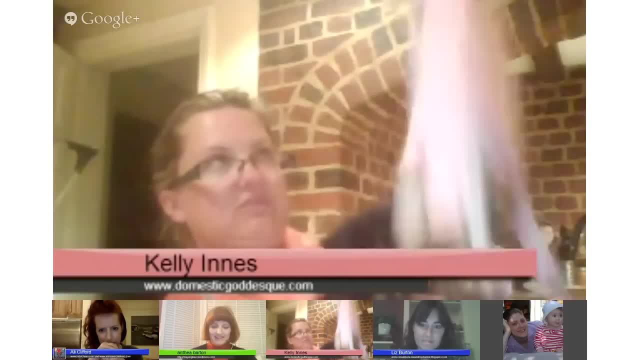 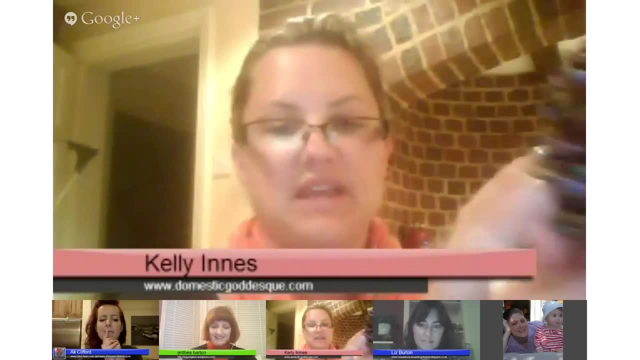 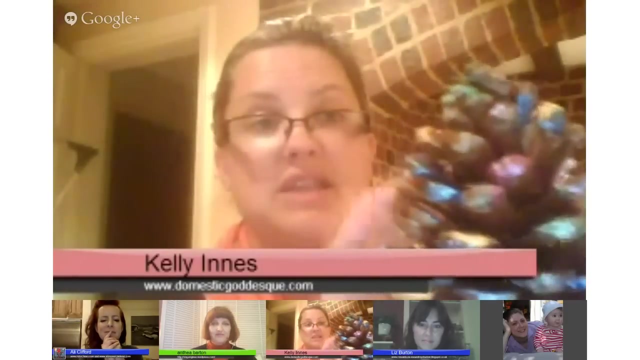 way, This is a pine cone wreath- well, a door hanging, I suppose What I like about this. I'll have to hold it up close to you now again, this is something I made with The girls and we well, really, I just left them to it. 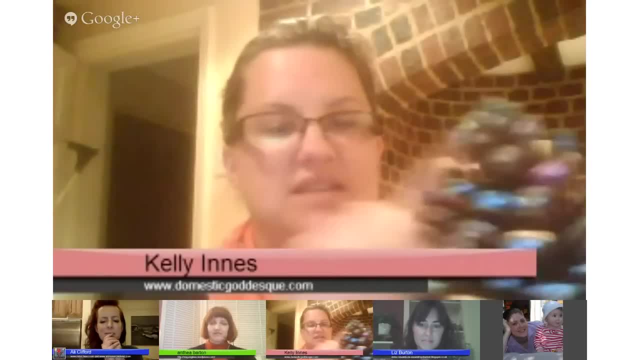 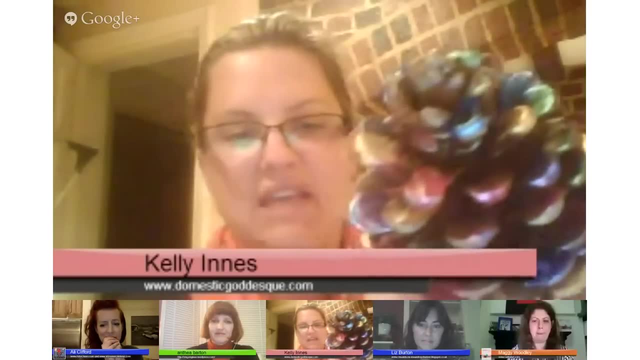 I gave them kind of a bunch of paints. These are metallic pastel paints, so there's blue, there's gold, there's pink, there's purple, And they had a go at painting kind of the little leaves of the pine cone. 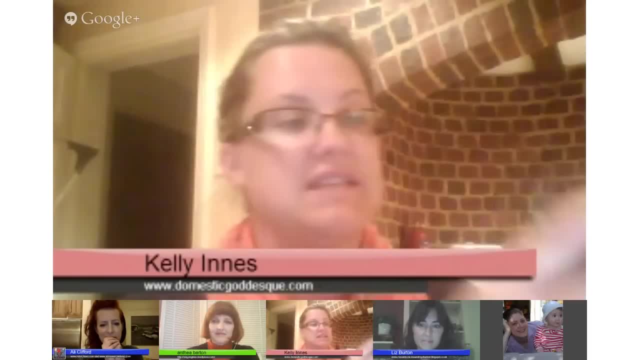 And they've just turned out to be the most beautiful things. I had them in a bowl for a long time and they kept disappearing into various handbags and push chairs And things around the house And I was terrified that I was going to lose them all. 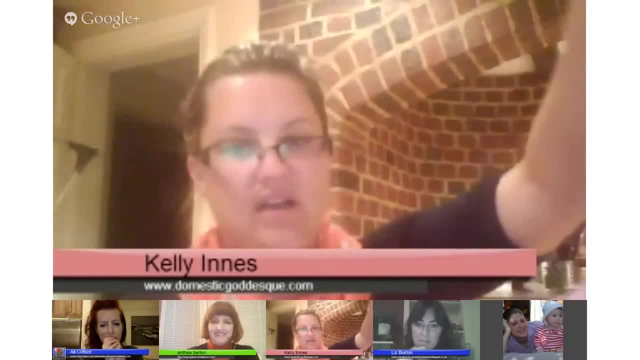 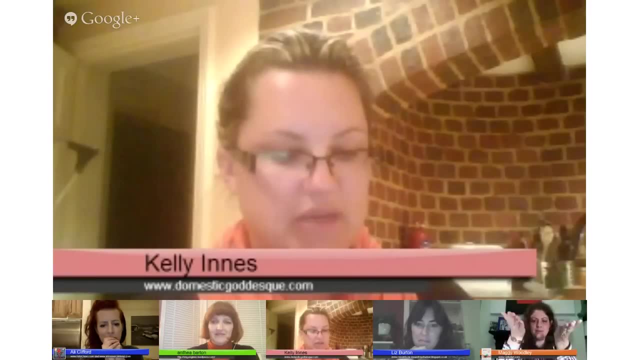 So I reclaimed them And, with the aid of a vast amount of ribbon and a glue gun- glue guns and burns go together- I made a door hanging. It's on the wreath, On the wreath. It's on the block. 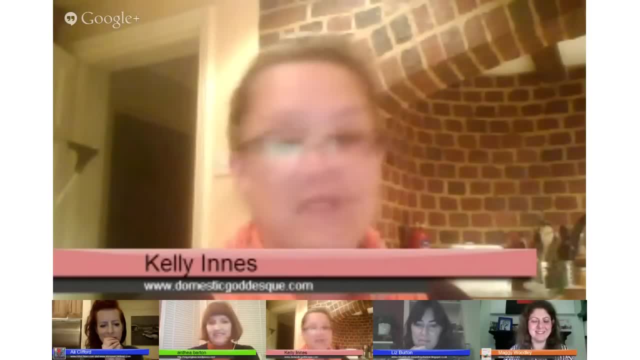 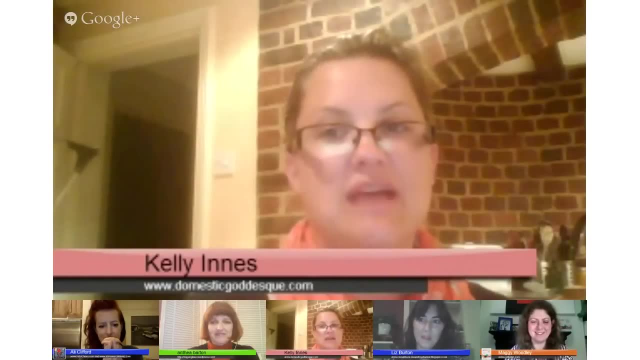 So you can see it there, But it has to be my most favorite nature craft, painting kind of thing. There you go. Anyway, I'm going to pass on to Lizzie, who hopefully will have a little bit of time to bring all this back to you. 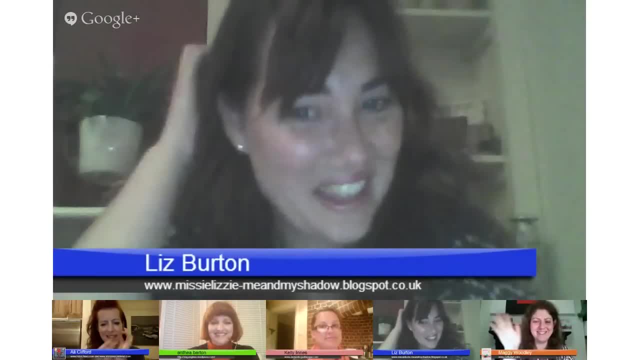 And they have to be beautiful. Just to say that this is a really beautiful cake, And the next thing I'd like to do- and I know we've been talking about this for quite a long time now- is make a pretty cat. I've seen it in a lot of different places and it looks absolutely gorgeous. 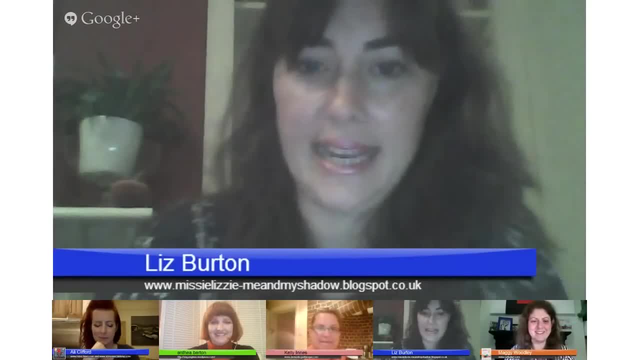 And it's really nice and gorgeous. I think it really is nice and it's beautiful. So we've got two ready to go. We have a big, small just to show you, and we've got a couple of other beautiful flowers that have come. 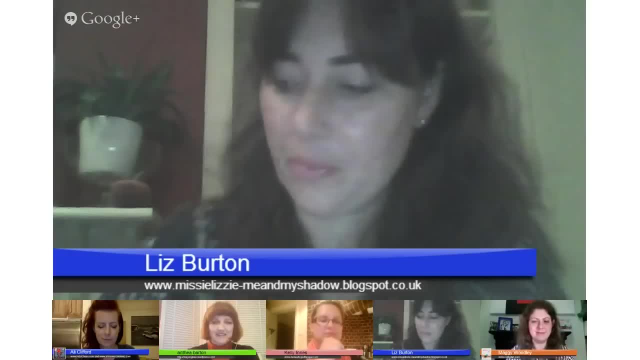 We've got two chocolate roses And they are beautiful, And these flowers are the ones that I am going to use for my decoration. These are some of my favourite decorations. I have a little bit of chocolate times and a little bit of purple for the background. 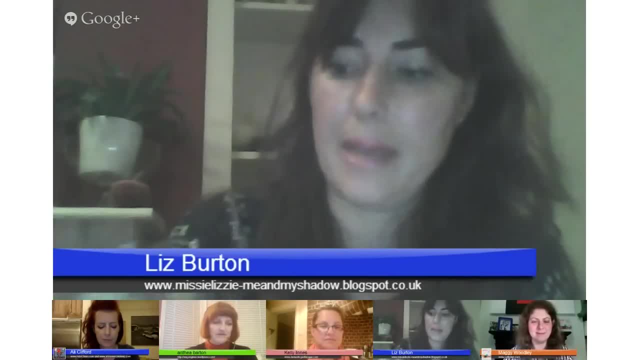 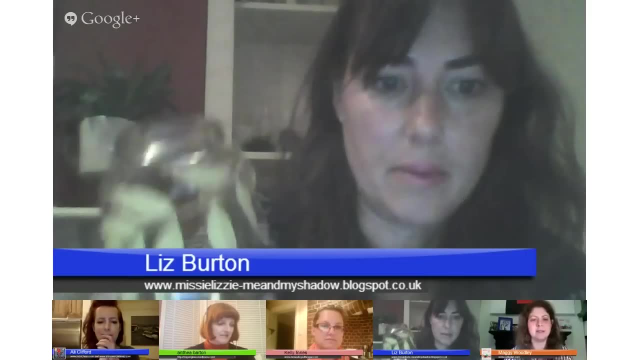 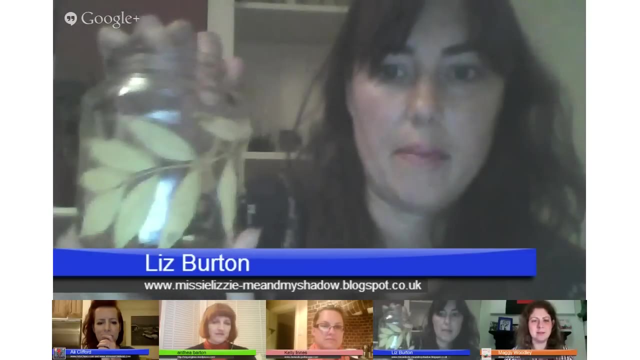 And for the background. Maggie's done similar with flowers and petals. but this is really simple, just basically hang on. I need to put me on big screen so I can't see what I'm doing. so this is just a leaf we picked up today on the way home from school and literally just hot glue gunned onto a. 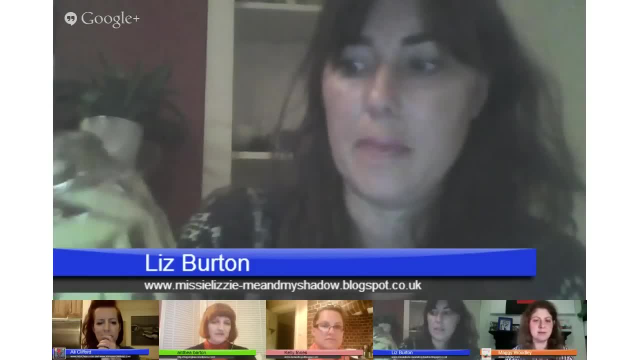 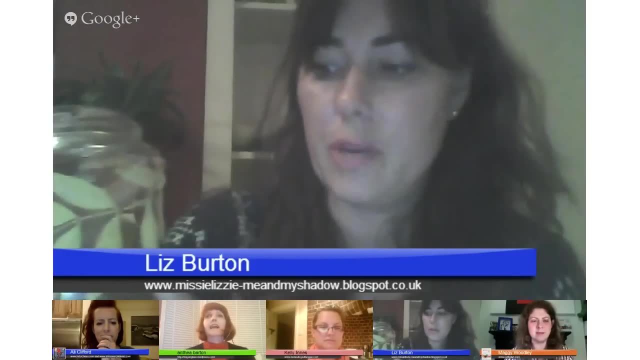 jam jar. so, and then with a little tea light candle in the middle, it just makes a really pretty table decoration. now, these obviously won't last forever. so what we'll do is, once we start getting the pretty colored leaves, then we'll dry them, stick them on and like: 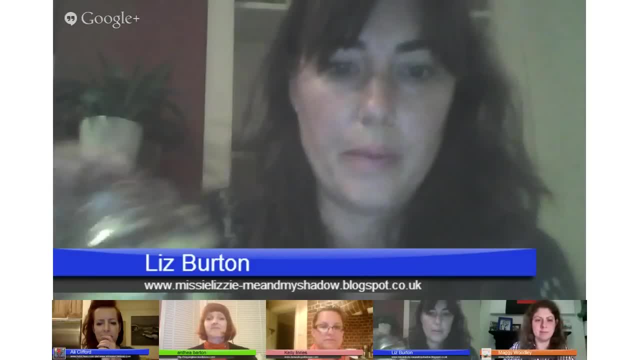 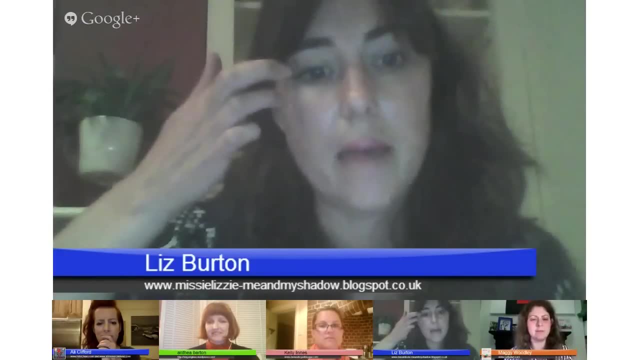 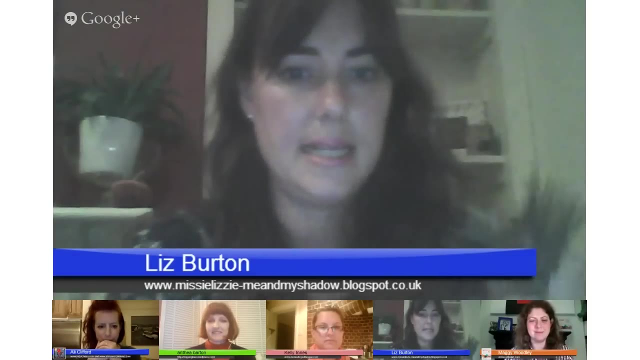 I think Maggie's done. before you mod podge or PVA, glue them and seal them on so they'll last a bit longer, but as a temporary thing you know really quick craft to do. it's nice, nice little display. and the other thing that my daughter's made is this. you can see him. 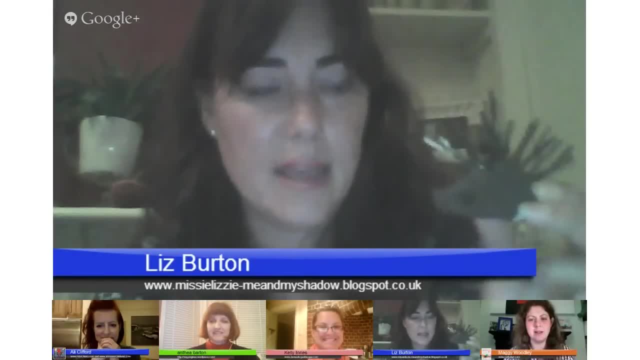 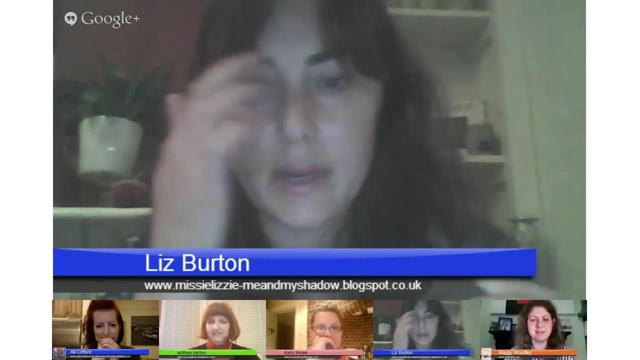 because I'm a bit dark and little hedgehog with sticks. so he's just made out of a blob of air dry clay which has been kind of shaped. shape the nose, use a pointy stick to make some eye holes and then you just go. I mean, kids are always gathering up sticks, so little. 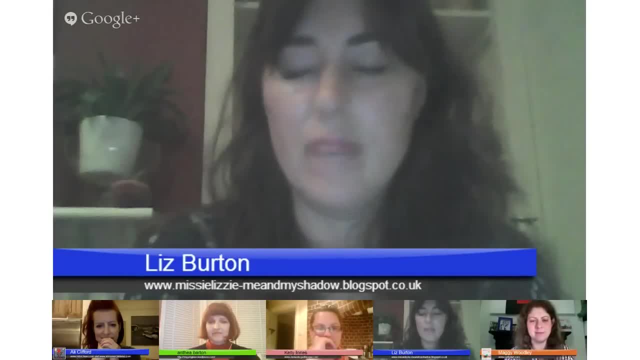 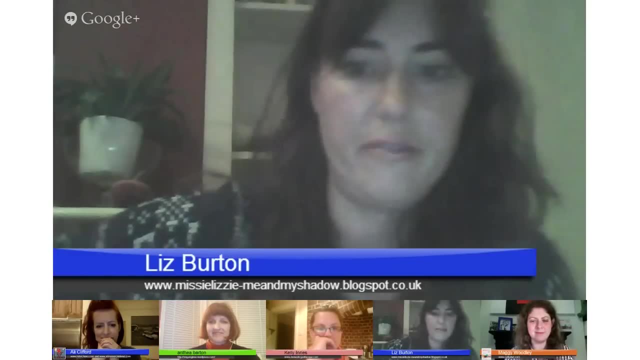 sticks poked in for the spines and then painted. so really, really simple thing to do. then this one I think I've shared before and it's on the blog, but again, if you're out and about in the woods, this is a really nice thing to look out for, if you can find any. 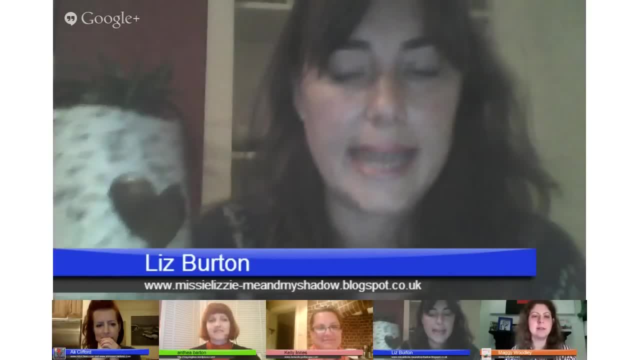 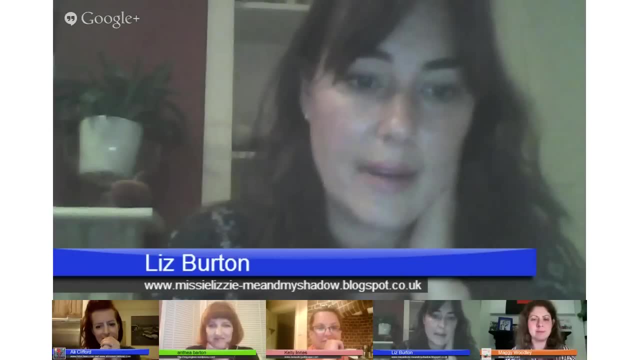 silver birch bark. you can't take it from a live tree, obviously, because that's very naughty, but very often with silver birch trees you'll see them laying on the floor with dead and decaying and you can literally just peel off bits of the bark. so you can check on the blog how to do this. you. 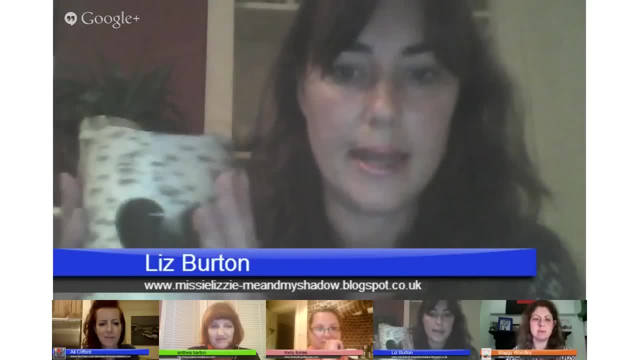 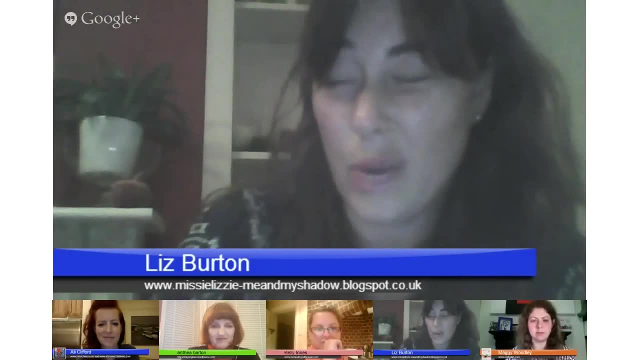 do need to soak it and stretch it and mold it while it's wet, and then it stays into position and then you can carve your shapes out. and that's that and the last thing I wanted to quickly show you, because I wanted to show you how to make a little bit of a little bit of a nice little. 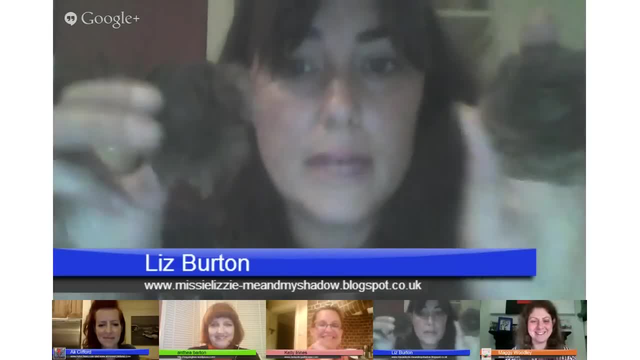 shape with your hands and I think you can see that there's a little bit of a bit of a little bit of a want, some ideas. ladies, are these beautiful little- I don't know if you can see them- these pine cones that look like roses? And I was trying to figure out what tree they 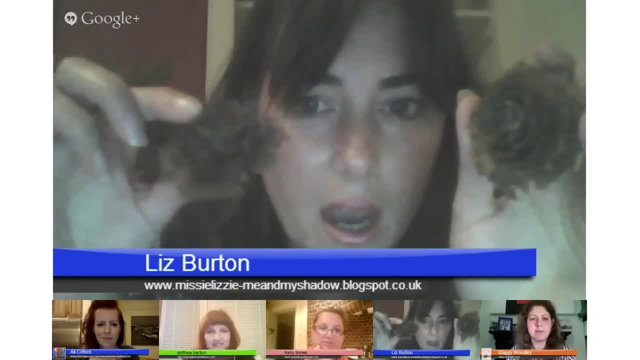 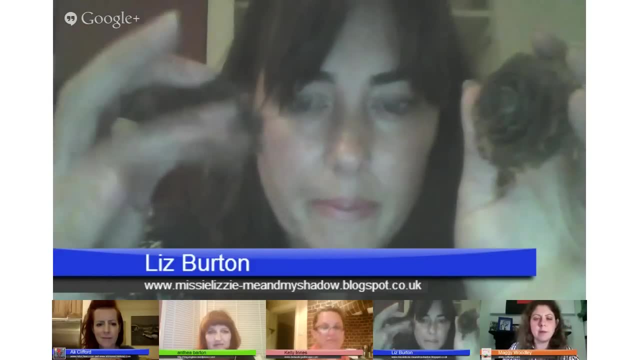 came from. It's some kind of cedar tree, But they're really lovely And I'm thinking I might be able to, like Kelly did, just paint the little you know, highlight the little petals, as it were. We get those near us, Liz. They're lovely, aren't they? I don't know, It is a cedar tree. 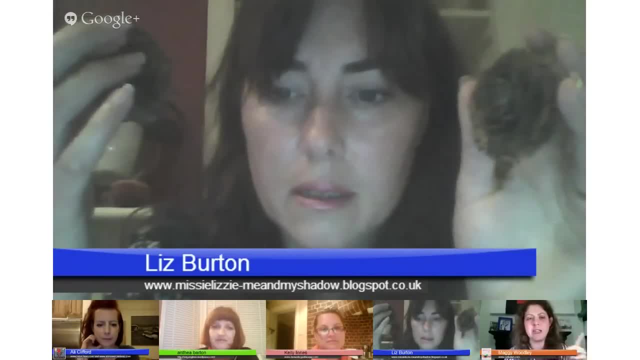 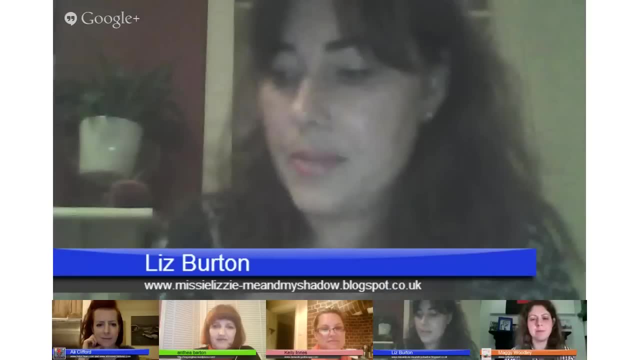 definitely, It's a type of pine cone, But I don't know what it is, But we have one tree in a park near us that has them, And I'm forever picking them up. They're beautiful, aren't they? They're beautiful. I think I could make a big wreath with them. So, anyway, I like those. 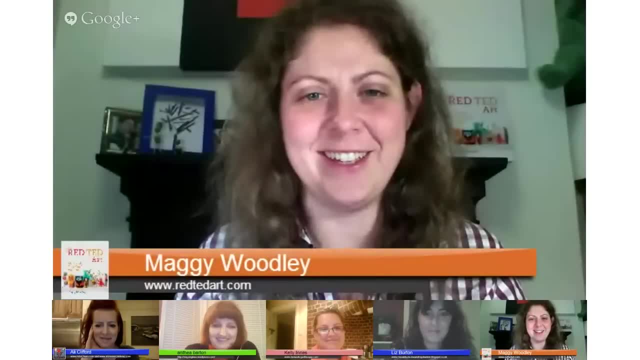 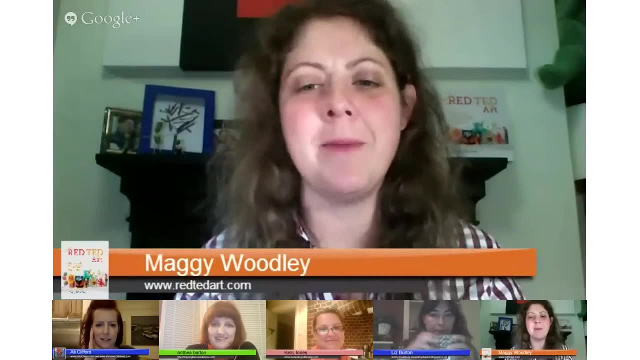 Anyway, that's me. I'll hand you back to Maggie Lovely, Thank you. I hope we haven't been experiencing connection problems. It just seems to be a bit funny today, So hopefully this is all going really well. I love that. 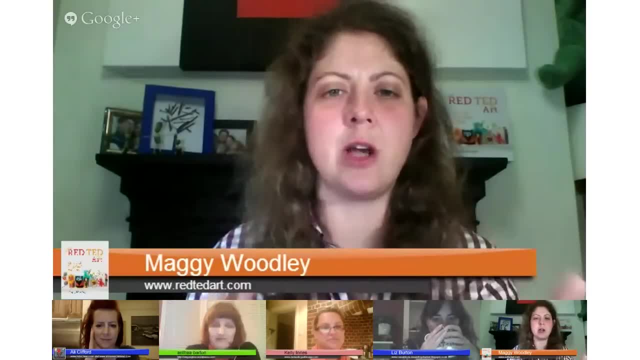 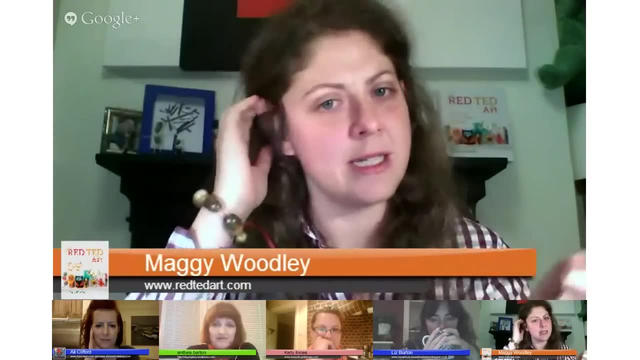 Liz has just shown us those little roses, Because what sort of this nature hangout is about is looking what you can find in your area, And obviously we're not all going to go out there and find these little roses now, And it's a coincidence that I know of a tree near us that does have one, But it's. 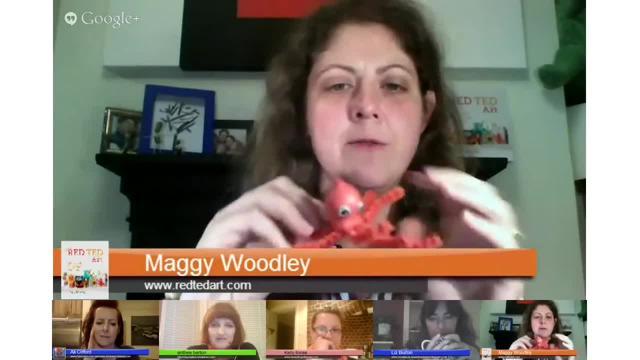 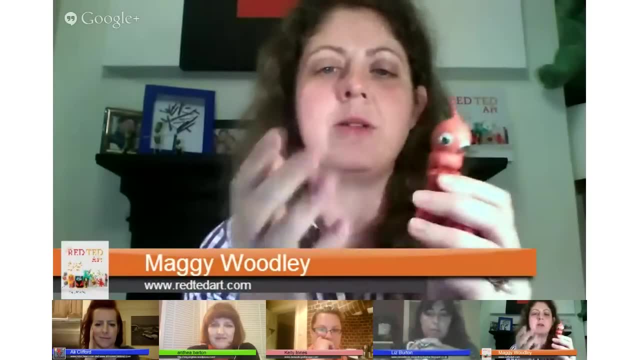 about having a look at what you've got in your area. So, for example, I did these especially for my Australian friends. These are gum nuts And I wanted to make sure that I had a few crafts with the gum nut thing, whatever you want to call it. And this is a pencil topper. 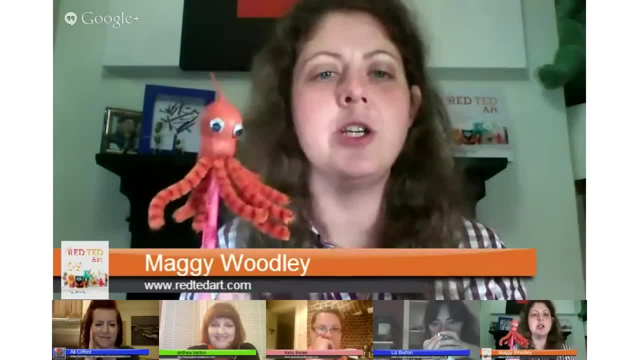 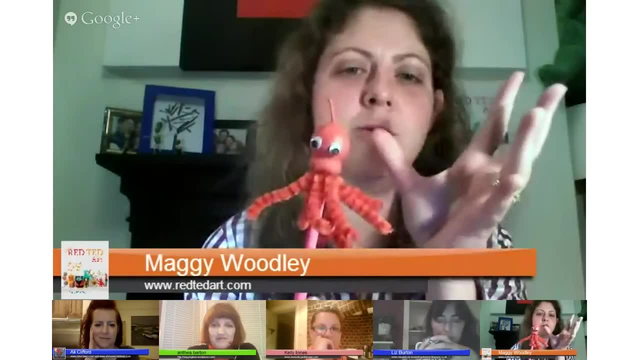 So you can put it at the bottom of the pencil. So it's finding things that are local to you and coming up with things. What does the shape remind you of? I just saw this and I thought: oh, it looks like an octopus. 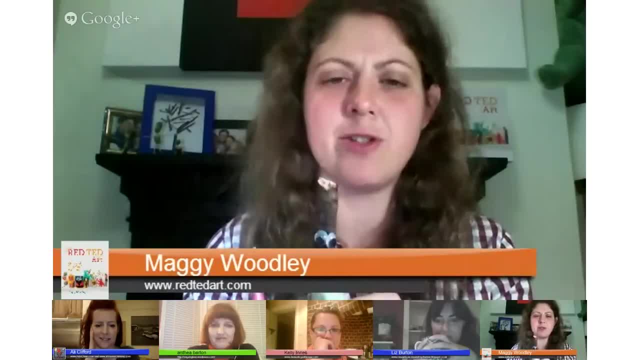 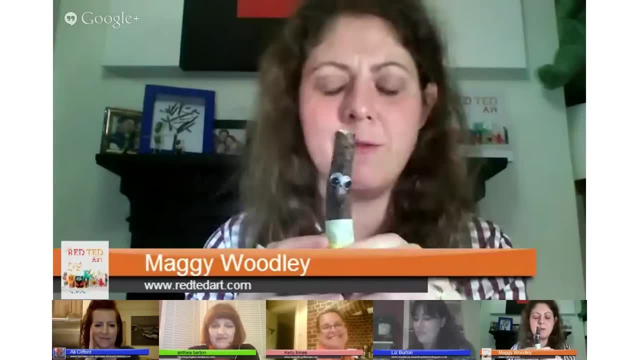 So what does the shape remind you of? What could you do? One of my favorites, really simple crafts, the stick men, Although I have to say I rather like the idea of Kelly's little fairy with the leaf wings and everything. Kelly, I reckon what you should also do is 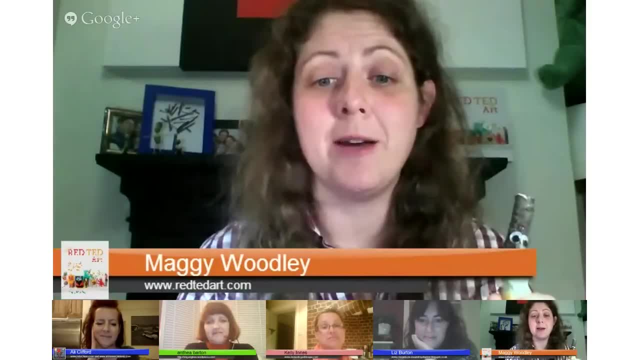 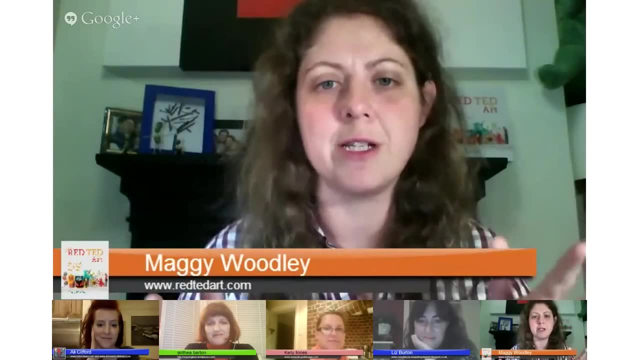 do a little fairy house for your fairies at the bottom of a tree. We love making them And what I always tell the children is: you have to make it with local materials, because it's a local fairy. So when we went to Austria, we had little maze leaves and little flowers. 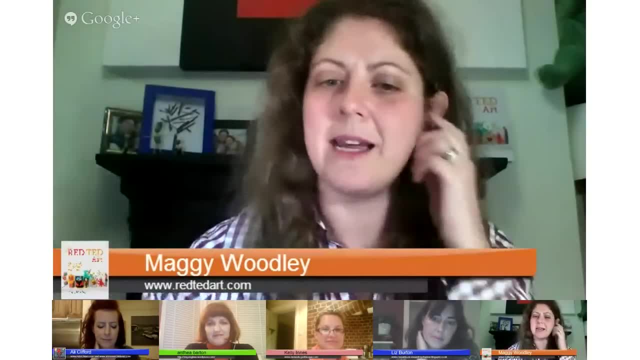 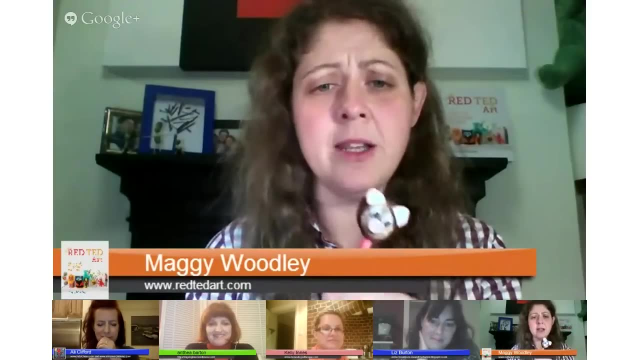 that were local. When we were in Spain we did it with the local plants there And if you've got such a big garden it's a perfect opportunity to do a little fairy house to ward off those naughty badgers. Another quick one, to like it: Little pencil, again pencil. 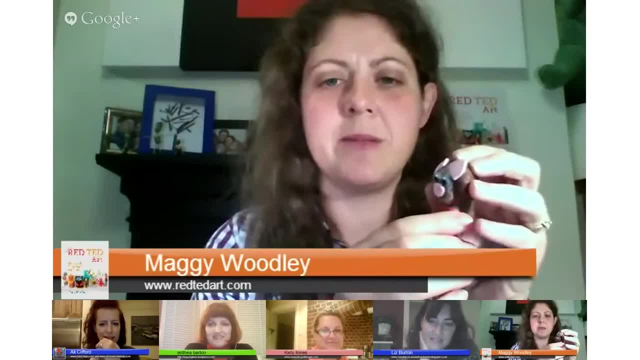 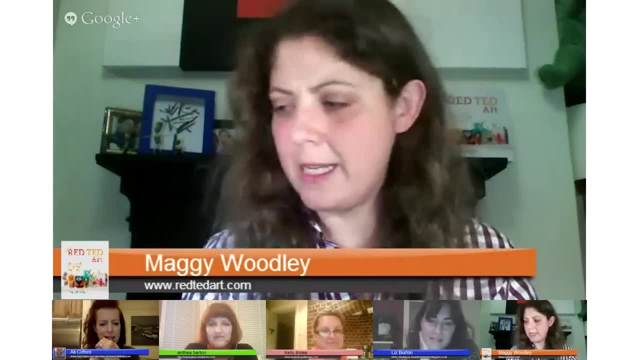 topper made from a chestnut. Chestnuts tend to shrink over time, So some people don't like crafting with them so much, But this one shrunk and it still works, And I think it's really sweet. It's on the blog. And then, what can I tempt you with? Oh, what I wanted. 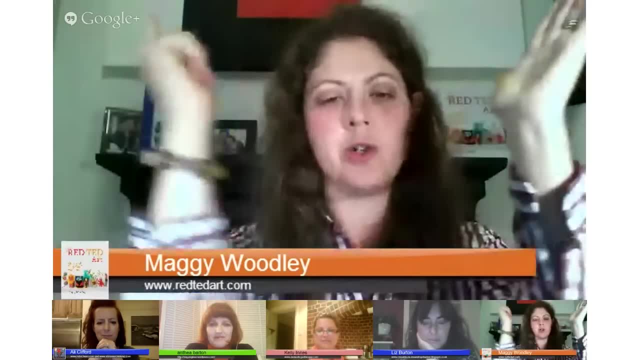 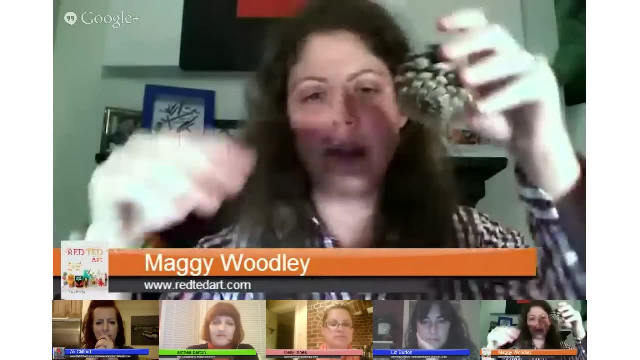 to say about antheas, With your branch, with the wool. it could be really nice to display lots of nature items you found, Because in the past I've taken all these things and made this big, huge mobile that we've hung from the ceiling And it's a really nice way of kind of making it an. 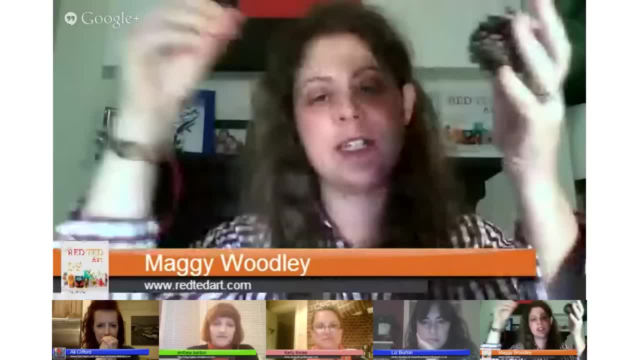 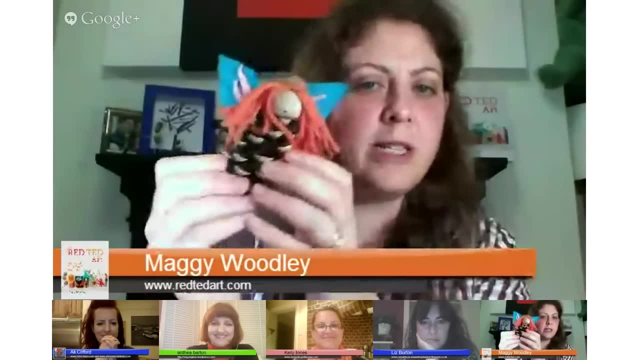 autumn-y feel, But I quite like the idea of your fork and just sticking in feathers and other things that you find as you go along, So all sorts of things. Here's another one. We're going to link all these things up at the end, But there's lots. 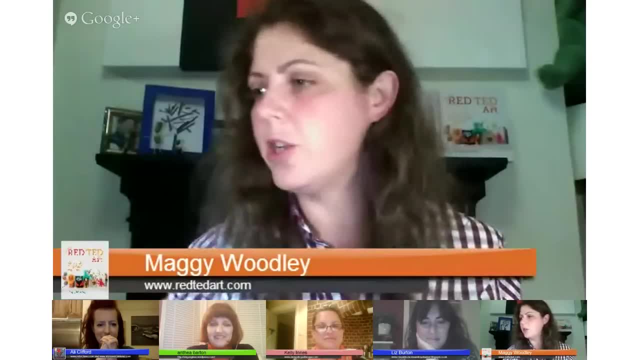 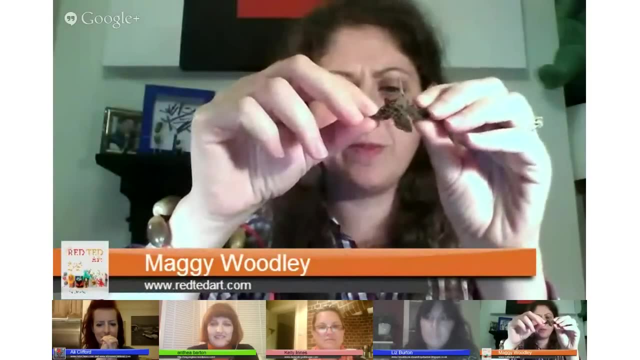 of different things you can do in autumn, And the main thing is that you go out there, that you look at shapes and you say: what does this remind me of? What are these called? again, Beech, Beech nuts, yeah.